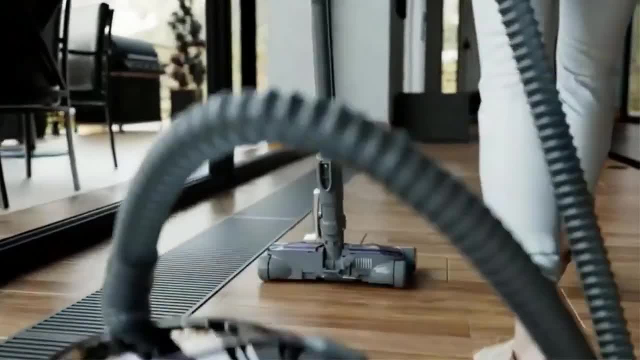 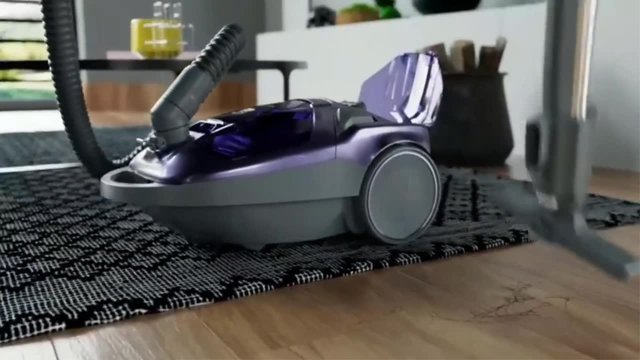 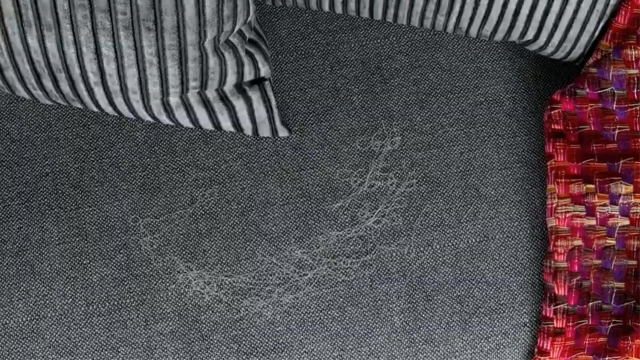 keep unwanted debris from escaping, and its haper filter on the exhaust makes it an excellent choice for those with pets or allergies. Along with assing our floor cleaning tests, our experts found the controls easy to use, and maneuvering was a breeze thanks to the big wheels. We loved that the floor brush can be. 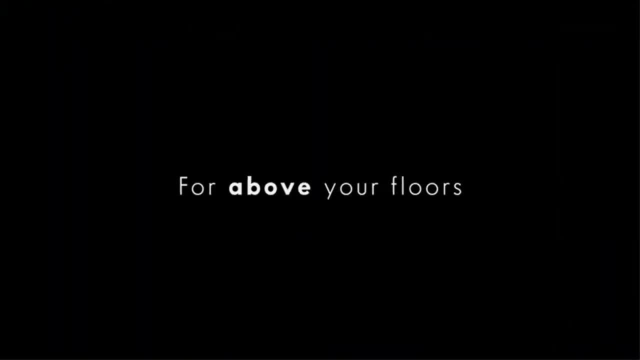 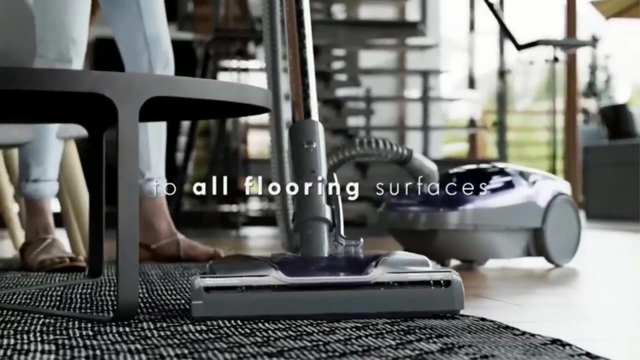 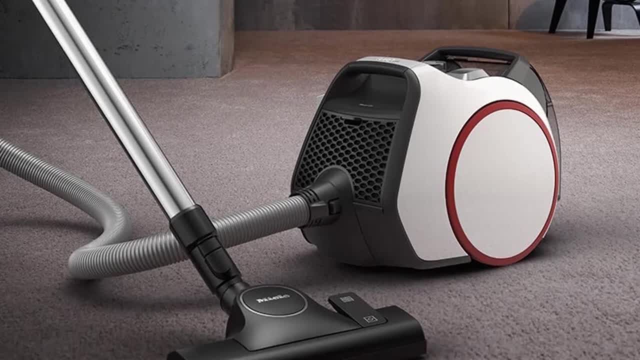 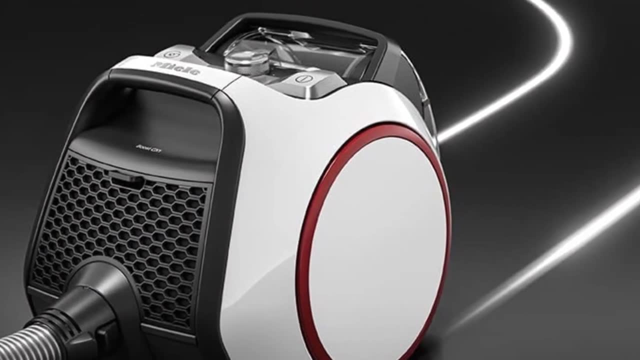 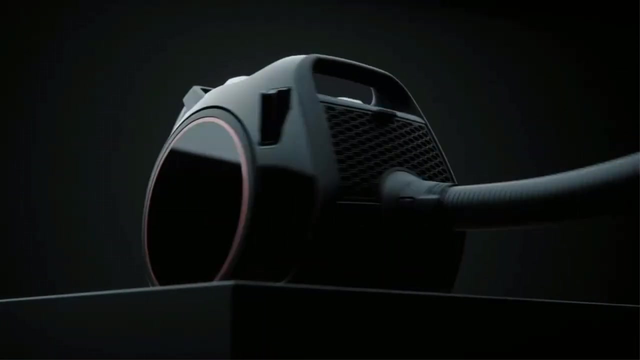 and the Boost CX-1 is no exception. With a sleek, compact design and flexible rubber hose, this canister vacuum impressed our experts in both the looks department and, more importantly, the performance department, earning a spot in our roundup of the best canister vacuums. 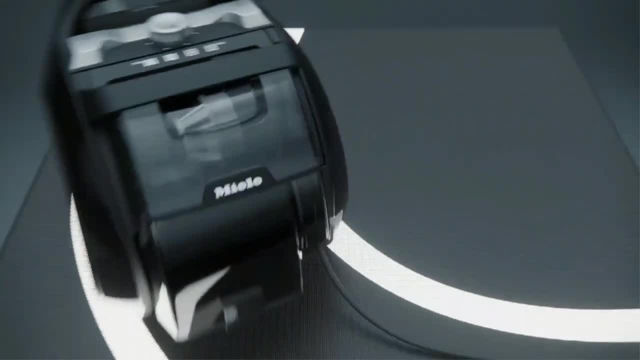 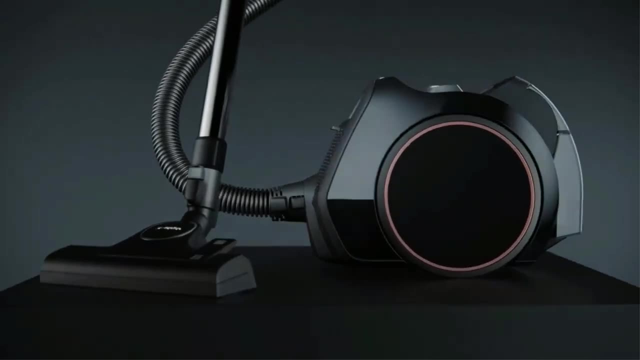 It picked up dry oats from all of our test floors and carpets with no problem and showed no signs of pushing debris forward instead of suctioning, which is a common complaint with other vacuum models, Thanks to a universal floor head that only requires the flip of one switch. 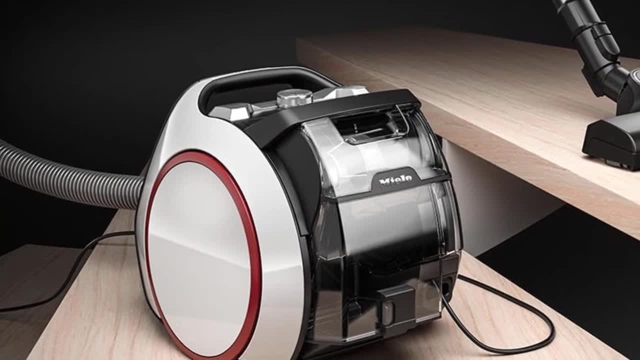 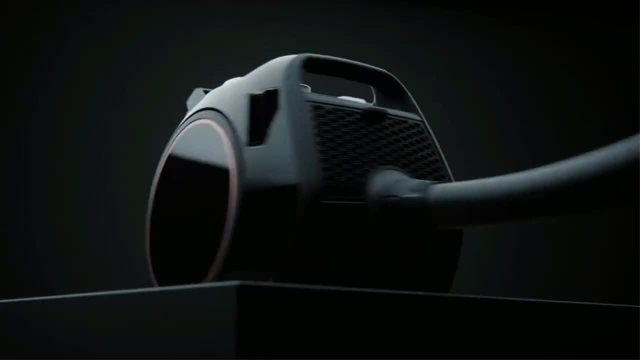 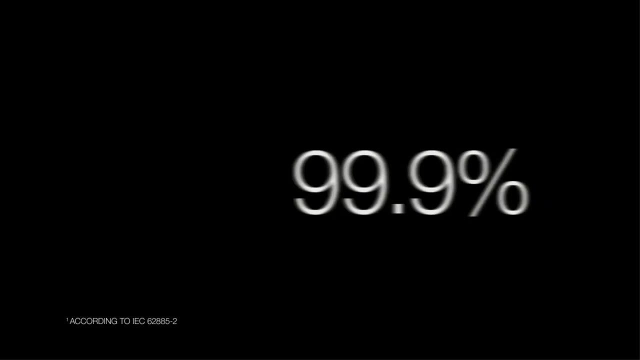 there's no need to change attachments when going from carpet to hardwood floors, But if you want to ensure your hardwood floors are getting the best treatment, the Miele comes with a parquet floor brush attachment for even better performance on hardwood flooring. The Boost CX-1 is bagless. 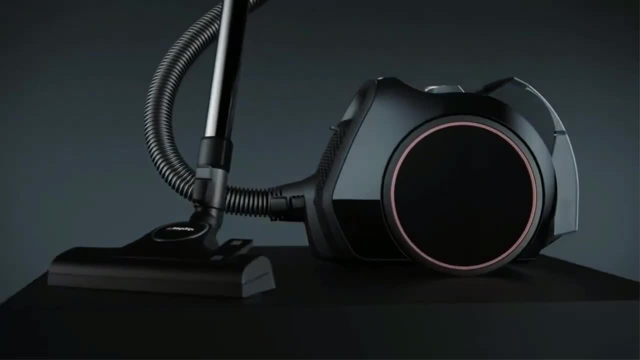 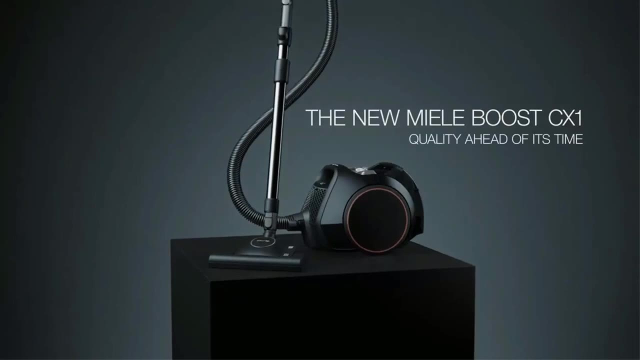 but with a Hygiene Air Clean filter that keeps even the smallest particles in the canister Allergy Suffering. Our testers can rest assured that they aren't releasing dust back into the air with this canister vacuum Number 4.. Hoover Complete Performance Canister Vacuum. 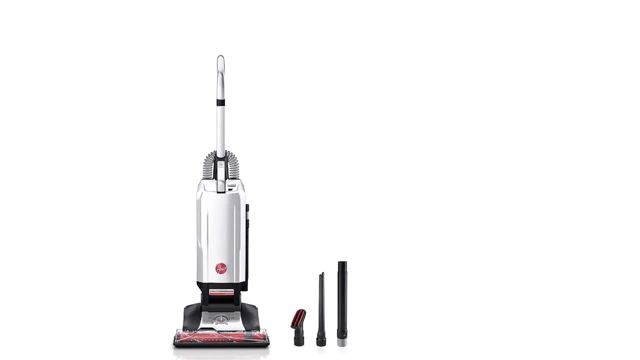 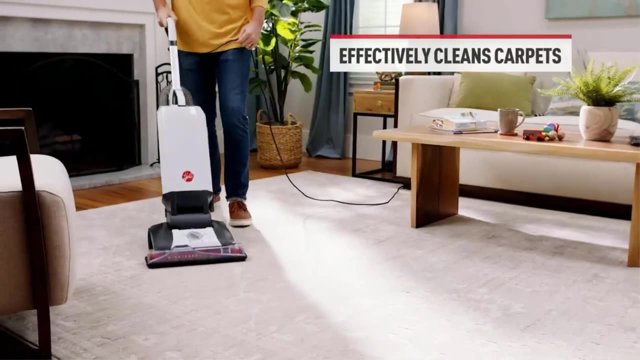 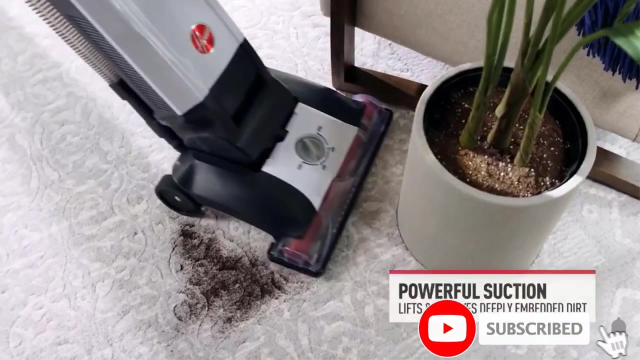 The Hoover Complete Performance Bagged Upright Vacuum Cleaner is an easy pick for our best upright option. Its effective performance in our lab and sturdy design are standout features. Our tester found that this Hoover model did a great job on hard floors, carpet and furniture alike, picking up debris and hair in just two parts. Our testers can rest assured that they aren't releasing dust back into the air with this canister vacuum cleaner, Number 5.. Plumbieter Vacuum Cleaner. This canister vacuum is a good product to use whenever you need to clean multiple floors. 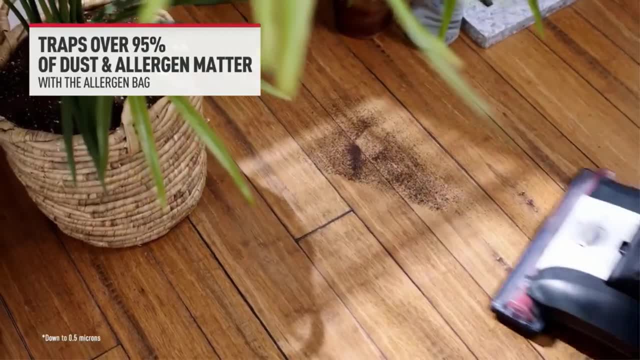 and to clean the main Fuel Changer. On the outside, the vacuum is designed to clean your whole bathroom. As we can see, the vacuum cleaner is a 15-inch cleaning path and a 25-foot power cord, so you'll likely be able to clean entire rooms without needing to change outlets. 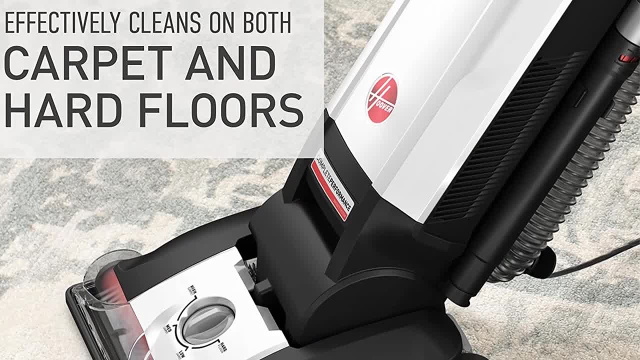 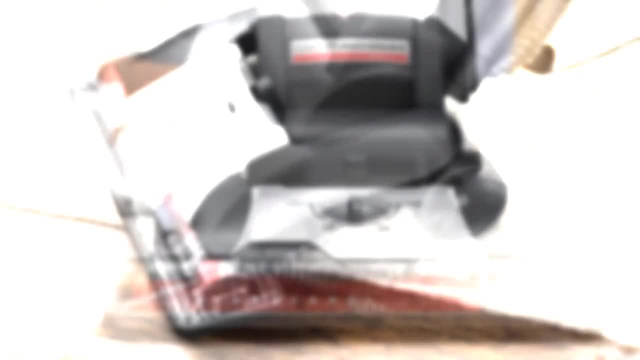 Notably, it's also both a bagged versus a bagless model. The bagged design, while not as seamless as a bagless one, is a benefit for those with allergies who don't want to be exposed to what they just suctioned up. However, if you don't like the idea of purchasing 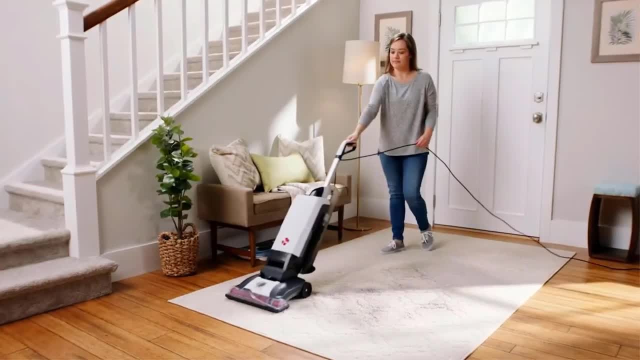 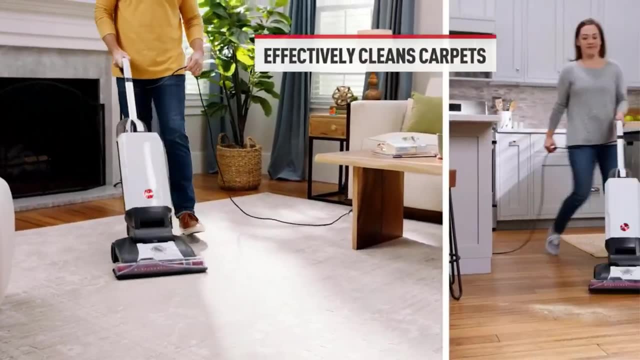 extra bags. you can always buy a going bag. Although the vacuum cleaner may be all for daily use, this design may not be for you. another potential downside is that, while this vacuum is efficient and sturdy, it features a slightly bulky design that requires extra effort on stairs and though. 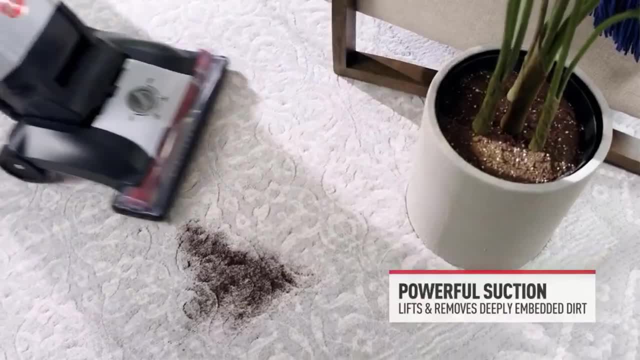 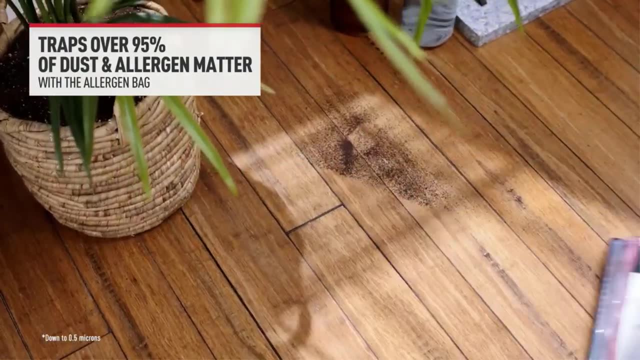 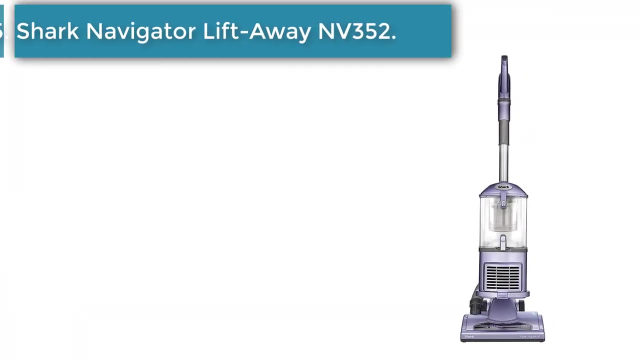 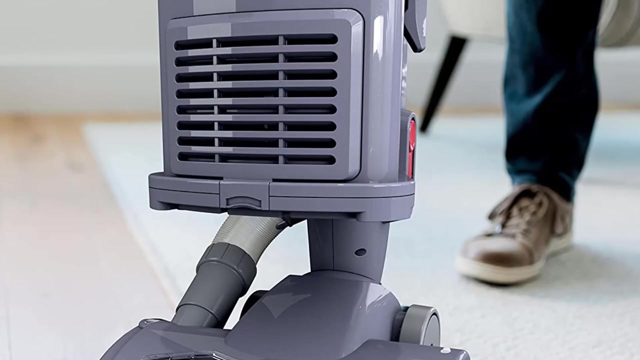 it does come with handy attachments like an extendable hose, pet hair brush and crevice tool. there's no additional tool for stairs. however, given its strong suction power displayed in the lab, we're still glad to recommend it for your hardwood floors. number five: shark navigator lift away- nv-352 canister vacuum. the shark navigator lift away nv-352 needs very little. 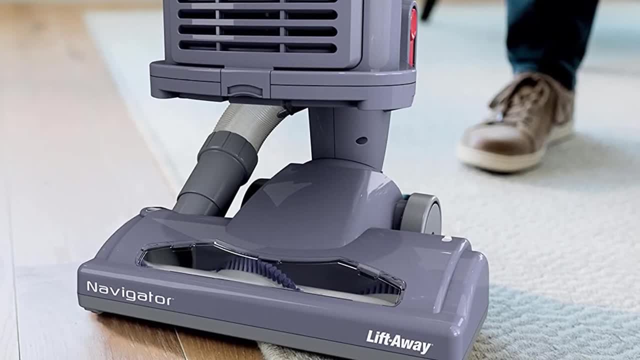 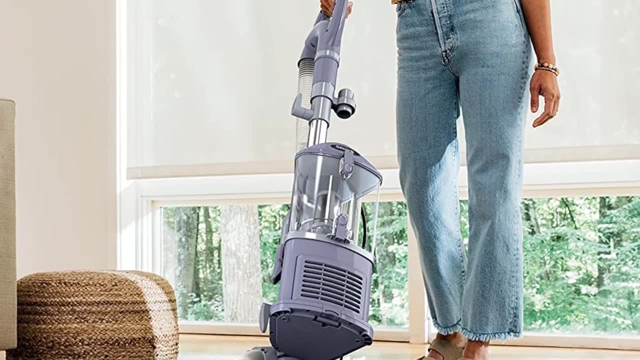 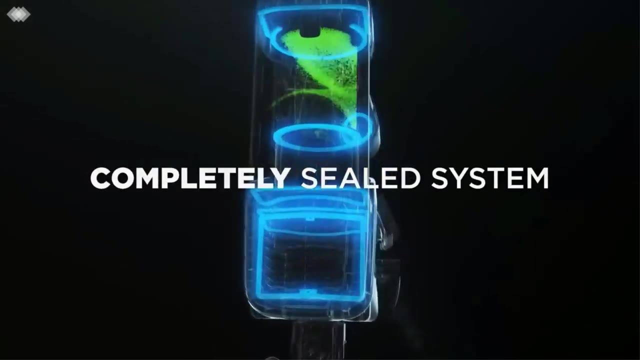 maintenance and has essentially no recurring costs. that's because its parts are made to last the lifetime of the machine, whereas most affordable vacuums need fresh filters and belts to keep running well. if something does break, shark's customers will have to be careful about that. service is generally good about honoring the five-year warranty. it's rare to see such an. 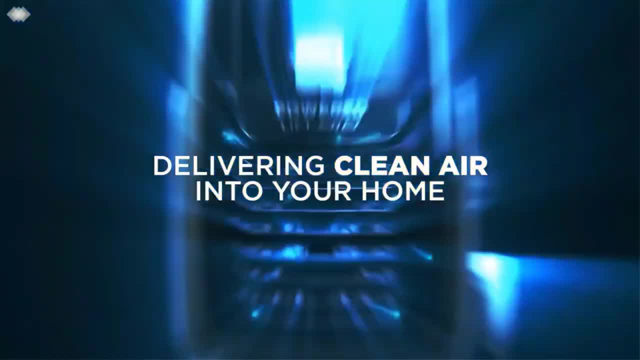 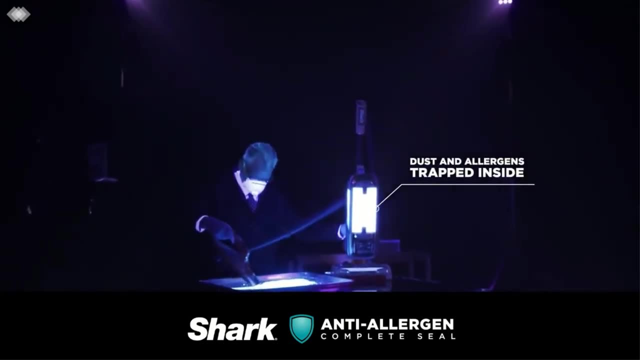 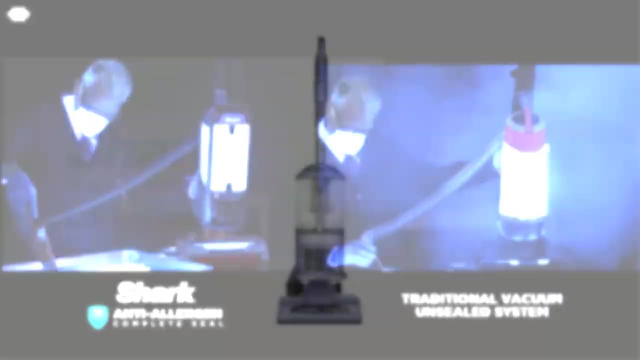 affordable vacuum backed by a policy that basically guarantees this kind of longevity. in our testing, we found the nv-352 to be a capable, well-rounded cleaner that can pick up all the typical types of debris- dust, crumbs, pet hair and more- from almost any kind of flooring.